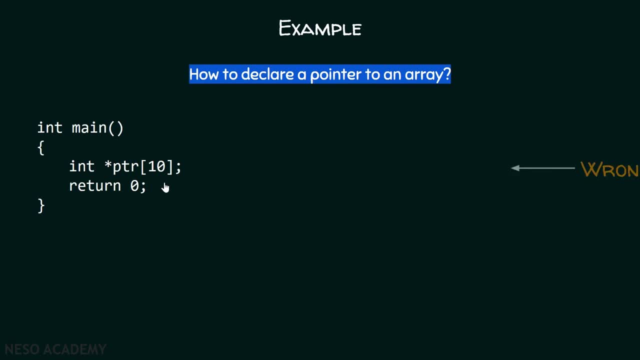 to declare a pointer to an array. But let me tell you this is wrong. This is not the right way of declaring a pointer to an array. This is an operand ptr. and here are the two operators. They are fighting with each other. 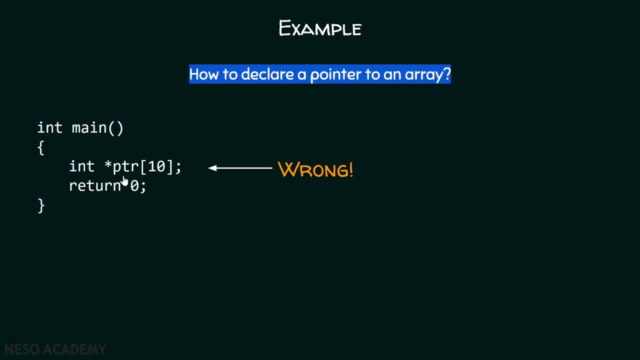 Square bracket says ptr belongs to me and star says ptr belongs to me. There is a fight between star and square brackets, But we need to eliminate this fight, and hence the precedence came into picture, Isn't that so? Always remember the precedence of operators. 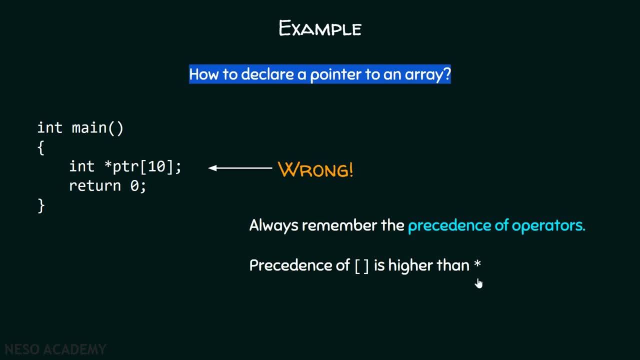 when such fight exists, Precedence of square brackets is higher than that of star. as precedence of square brackets is higher than that of star, Therefore square brackets wins in this case. Hence ptr belongs to square brackets. So we can say that ptr is an array. 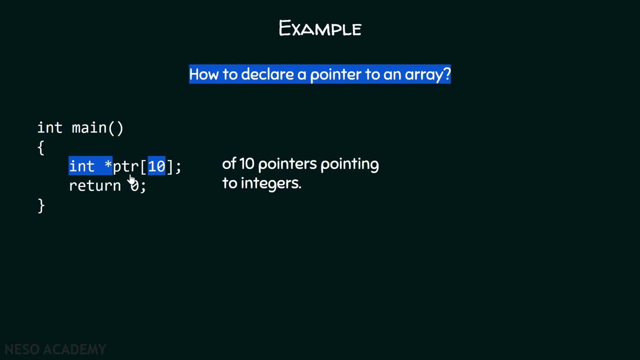 of ten integer pointers. Or we can say that ptr is an array of ten pointers pointing to integers. Okay, but what we want? We don't want an array that consists of pointers. We want a pointer which is pointing to an array. Isn't that so? 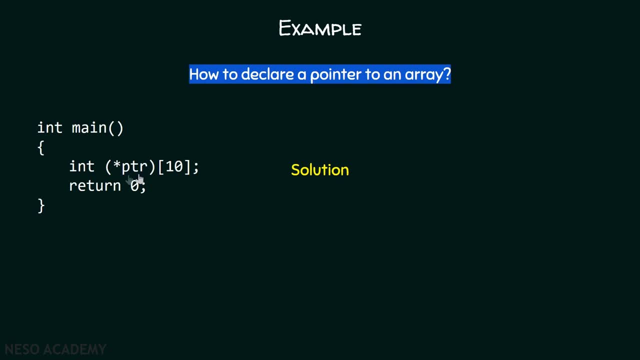 For this purpose, we will put these round brackets around this star, ptr. Why these round brackets have to be put So that the precedence of star becomes higher than that of square brackets. Then this star will belong to ptr, Isn't that so? 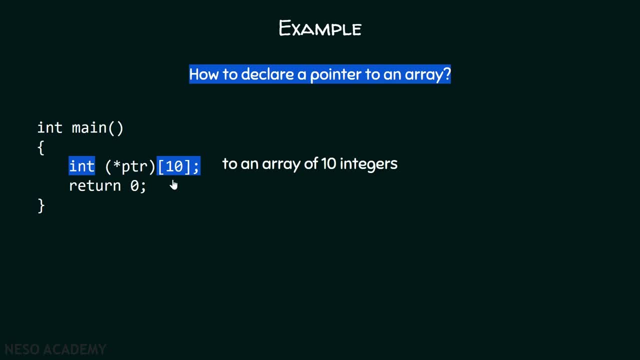 Star ptr means that ptr is a pointer which is pointing to ten integers, Or ptr is a pointer which is pointing to an array of ten integers. So this is the way we can declare a pointer to an array Here. in this case, this ptr is pointing to 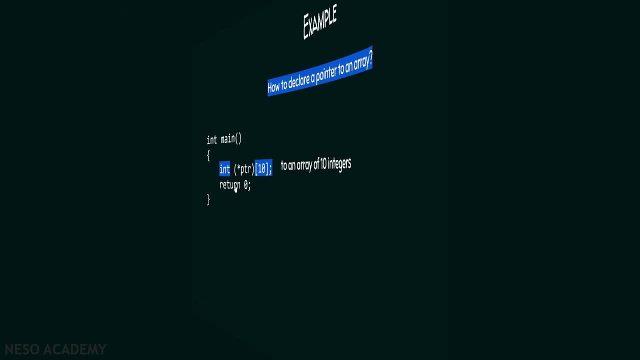 an array that consists of ten integers. Okay, fine. Now the question is how to declare a pointer to a function. then I want a pointer to the following function. This is the function add. We want to add these two integers, So we need a pointer to this function add. 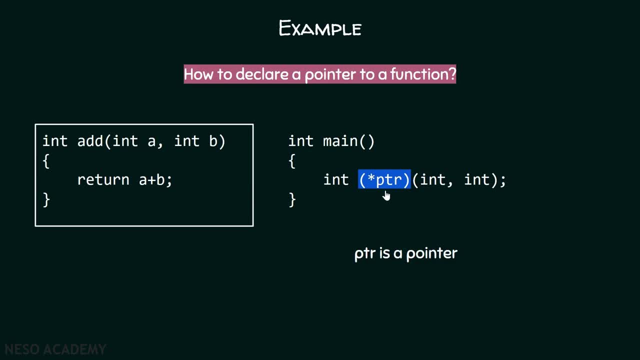 For this purpose, we can declare a pointer like this: ptr is a pointer which is pointing to a function containing two integer arguments and it returns an integer. Okay, so this is the prototype. So ptr is a pointer which is pointing to a function. 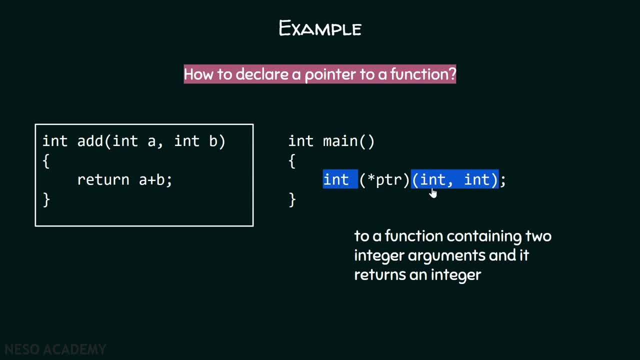 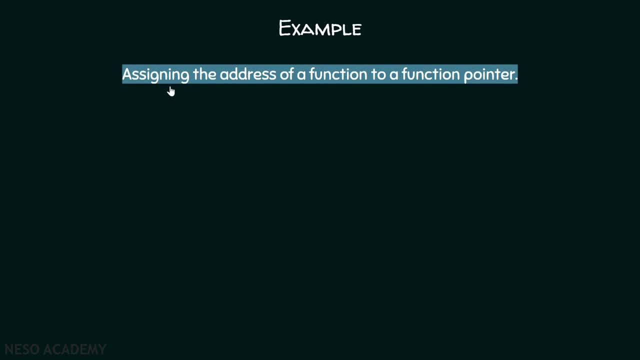 So this represents a function that consists of two integer arguments and it returns an integer. This prototype has to be remembered. Now let's learn how to assign the address of a function to a function pointer. Here is the function, and we want a pointer to this function. 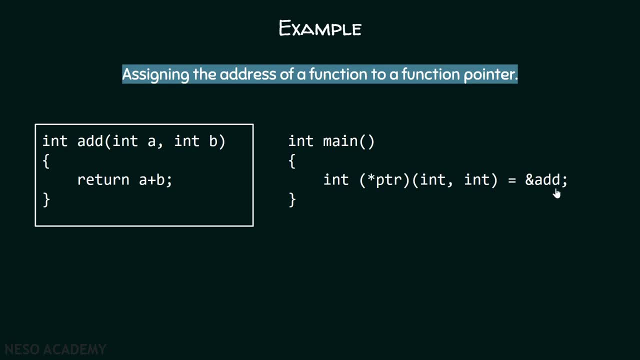 So for this purpose, we will simply assign ampersand of add. That means we will assign the address of this function to this pointer, Isn't that so? Or we can write something like this: The declaration separately and assignment separately. 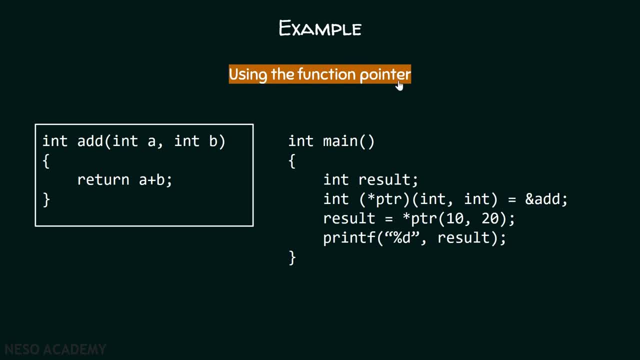 This can also be done. Now let's see how we can use the function pointers. After assigning the address of this function, we can use this pointer to call this function. Here we are using this pointer and we are passing the two arguments ten and twenty to this function. 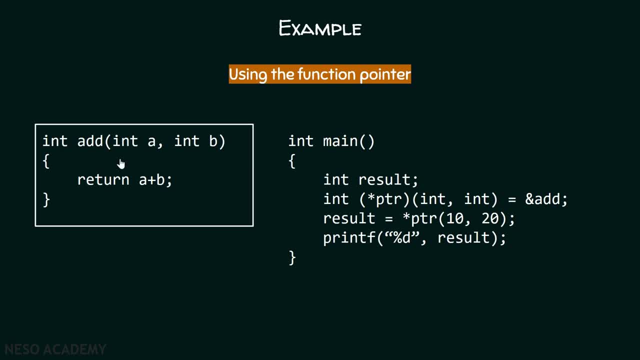 Because ptr contains the address of this function and now it can pass these two values, ten and twenty, to this function. After passing these two values, it will return some result. That is the addition of these two numbers, That is ten plus twenty, which is thirty. 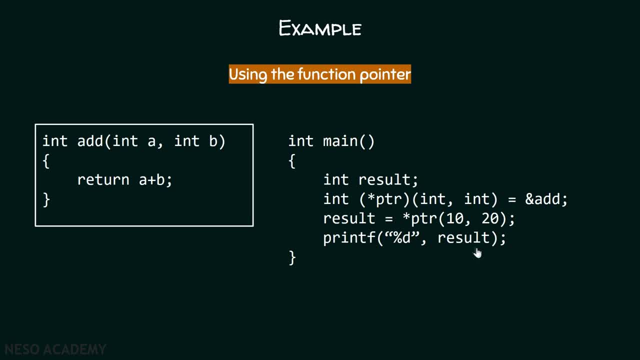 This result is now stored within this result variable and we can print this result on the screen. As simple as that. Or there is another way in which we can use function pointers Here: instead of passing ampersand add, we can also pass add, because 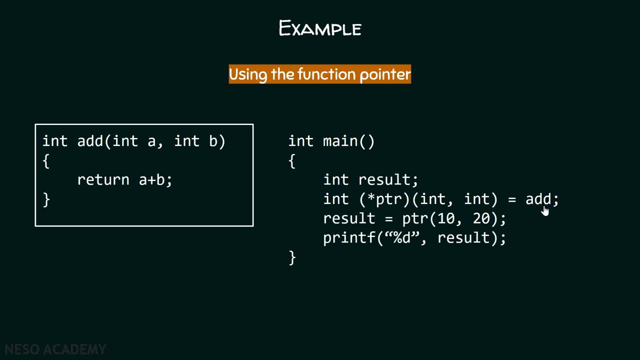 the name of the function represents the address of that function or the initial address of that function. So if we pass ampersand add or add, both are one and the same. Okay, When we write ampersand here, then we need to write dereference operator here as well. 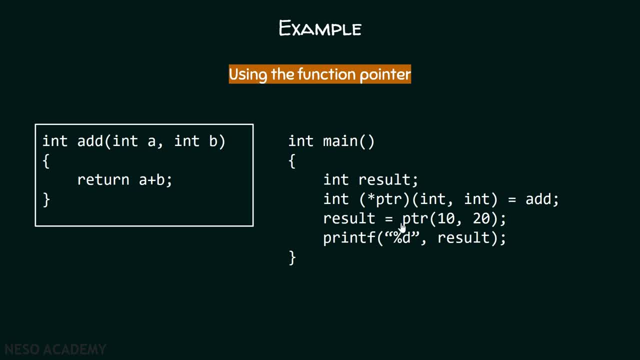 But if we didn't write ampersand here, then there is no need to put a dereference operator here. We can simply use ptr and pass these two arguments to this function and then the result can be returned and we can print that result on the screen. 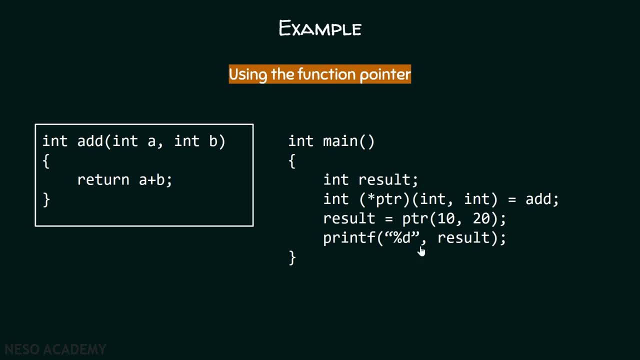 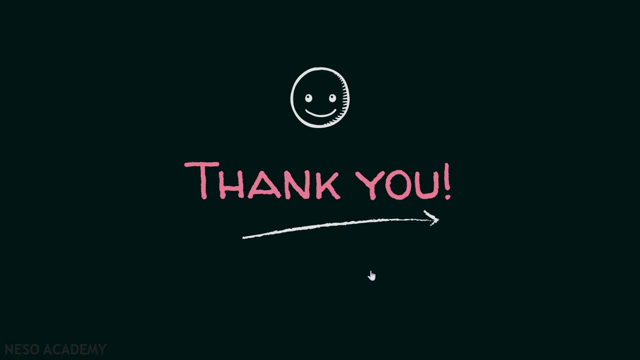 So this is much easier way of passing the address of a function to a pointer. Okay, Okay, friends, this is it for now. Thank you for watching this presentation.